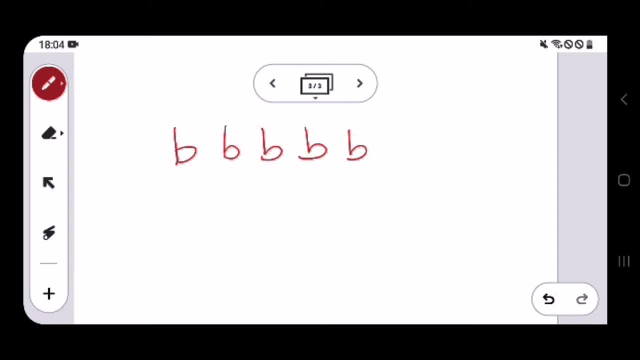 container here, and let's represent the containers by c1, c2 and c3. since they are all distinct containers, we can differentiate. So we know which is c1, we know which is c2 and we know which is c3.. Alright, so we have these 5 identical balls and we have 3 distinct boxes. Okay, so now let's say: 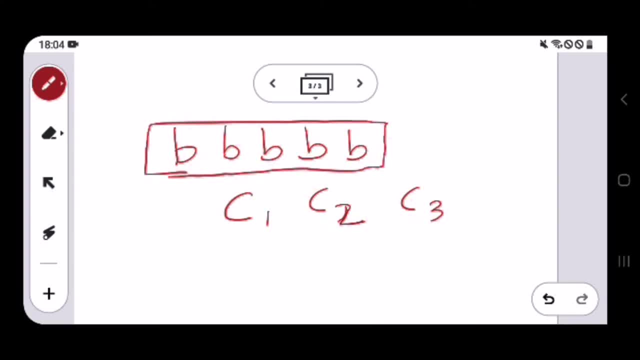 that we want to distribute into these 3 distinct containers. Okay, and how many ways can we do that? that is a question, Okay. so let's think about from the containers perspective. Okay, so here we have these 3 containers and c1 can have 0 balls. that is a possibility, right. One way of distributing that. 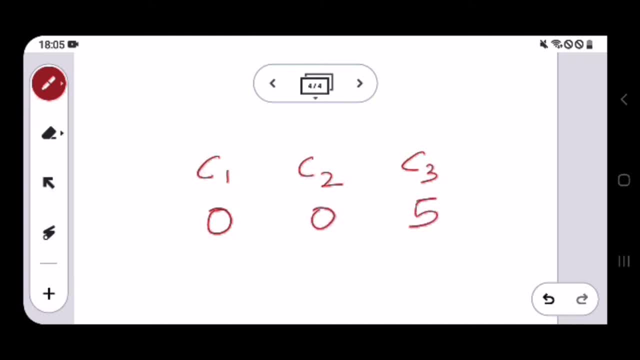 is a possibility, right. One way of distributing that is a possibility, right. One way of distributing these 5 identical balls is that one of these 5 can go to c3 container and c2 and c1 get none. This is one possibility right Now. okay, so let's understand it this way. So let's say that, since there are 3, 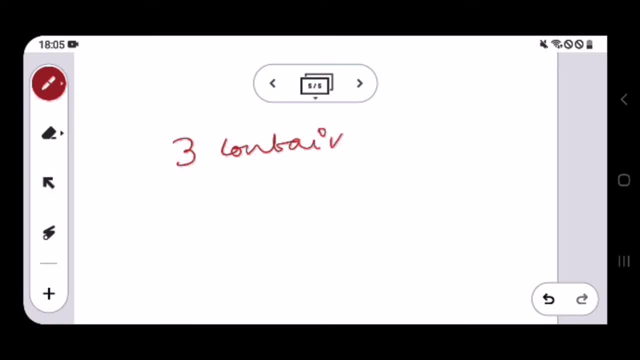 containers. right, what we will do is we will take 3 minus 1, which is 2 bars. Okay, so 2 bars. I will draw such that it will say it will distinguish these 3 containers. So the first bar here, whatever is coming to the left of it, is whatever is coming to the left of this bar. that much balls c1 has. 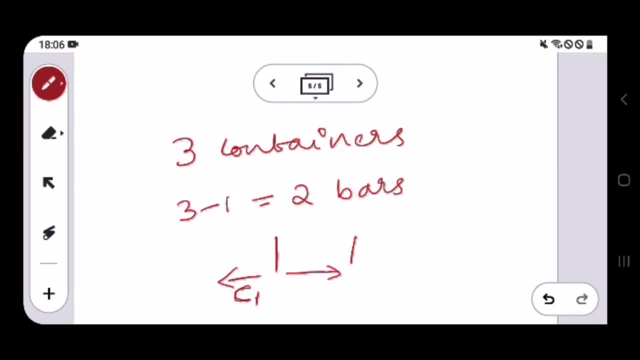 Okay, and in between the first bar and second bar, whatever balls, let's say, are there, that is in c2, and whatever is coming to the right of the second bar, let's say, that is c3 container, right, okay. and we have 5 b right, we have 5 identical balls. that is all 5 b right. Now it can come anywhere, right. 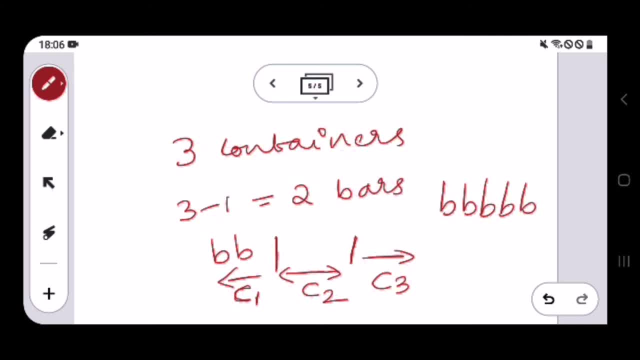 So one possible arrangement is like this: right, So 2 balls in c1,, 2 balls in c2 and 1 ball in c3. right and so in this way, the earlier example how we can denote this- c1 is 0, means whatever is left to the first bar is 0. So there is no b here left to this first bar, and we have. 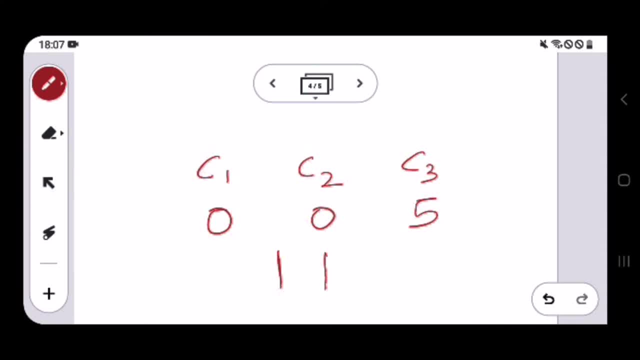 also second bar. So in between first and second bar is a place for c2.. Since c2 is 0, there is no b here Now. so to the right of second bar, we have 5 b, which represents c3. have 5 balls right. So this is how. 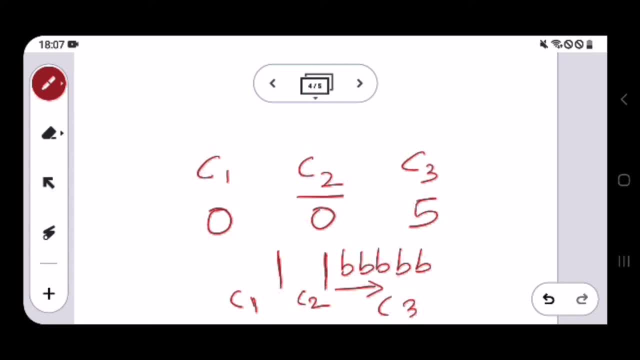 this is an arrangement. Okay so, this is an arrangement having 5 b and 2 bars. Okay, so there are 2 bars and 5 b's, right, and it's any arrangement of these 2 bars and 5 b is a distribution right. You can think about it, right? Any arrangement. 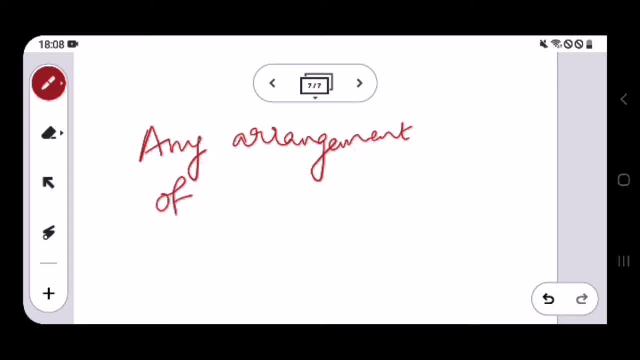 of 3 minus 1, which is 2 bars. any arrangement of 2 bars and 5 b's right corresponds to a distribution right. So how many distributions will be there? Well, it depends on how many arrangements we can have with 2 bars and 5b's. So we have the symbols Like 2 bars are thereand 5 b's are there. How many ways can we arrange this? that is the question. How many ways can we do that? See, a total of 7 symbols are there right? So 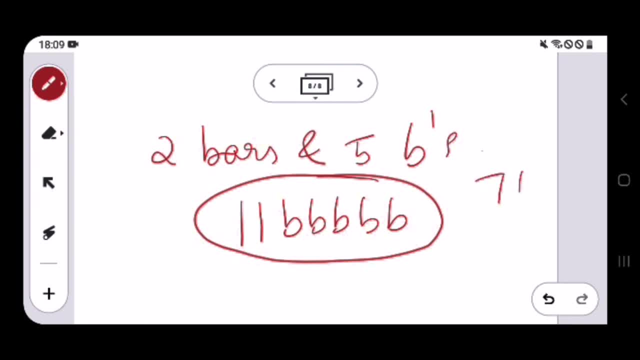 7 symbols, So 7 factorial by b is repeating five times, so by five factorial and bar is repeating two times, so by five factorial or two factorial. these many arrangements it can have right. in another words, how can we write it in terms of combination? this is in terms of permutation. we wrote right. so if in terms of 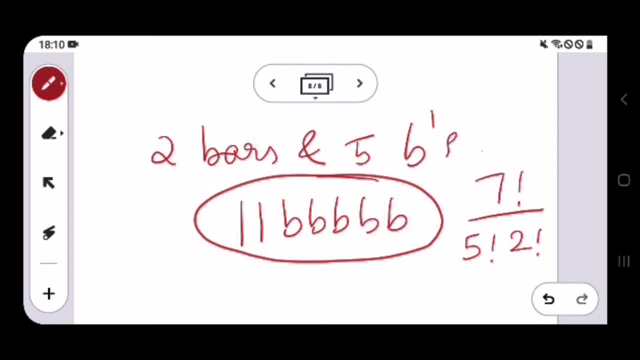 combination we want to write. we can just select the positions where the five b's goes right or two bars goes. both are same. if you just select the places where two bars come right, then if you just select the positions, okay, then automatically see there are seven positions. 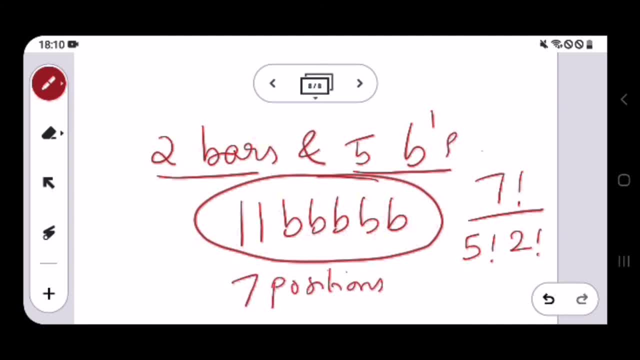 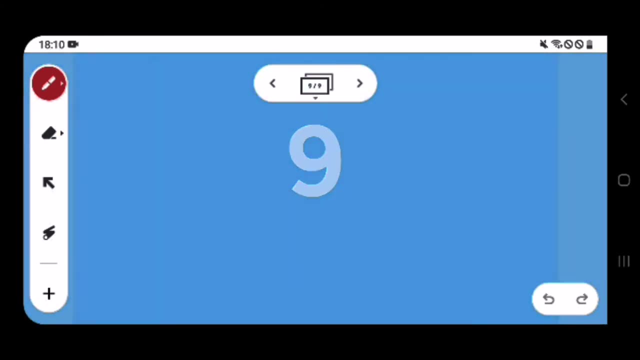 right. so here we have seven positions. so in this example, first position is a bar, second position is a bar right, and if you select these two positions for this bar, then rest of the places automatically b will come. okay, so combinatorially writing it is: seven choose five, which is same as seven choose two. 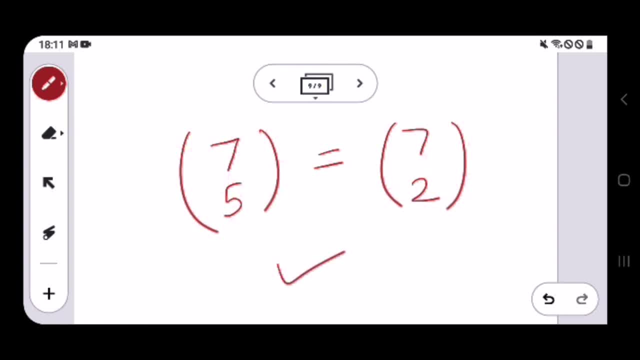 so and we got the answer actually. so we got the answer of the question: how many ways are there to distribute five identical objects into three distinct containers or boxes, whatever? okay, so now let's generalize this concept. now we have, let's say, n identical objects. see, these identical objects need not be balls always. i just took it for an. 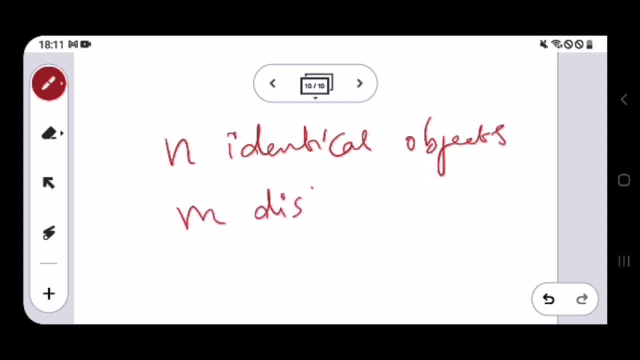 example. okay, and there are m distinct containers, right? okay, see, these m distinct containers: m minus one bars. we can have to distinguish between the containers, right? so? m minus one. so first bar left to the first bar, meaning that it is the first container. how many containers are there? there are m containers, okay, so 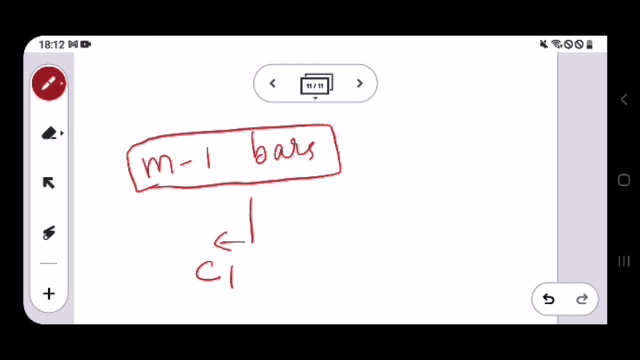 m minus one bars are needed. right, because left to the first bar is the first container, between the first and second bar is the second container, between the second and third bar is the third container, and so on. and after the m minus 1th bar, this is m minus 1th bar. 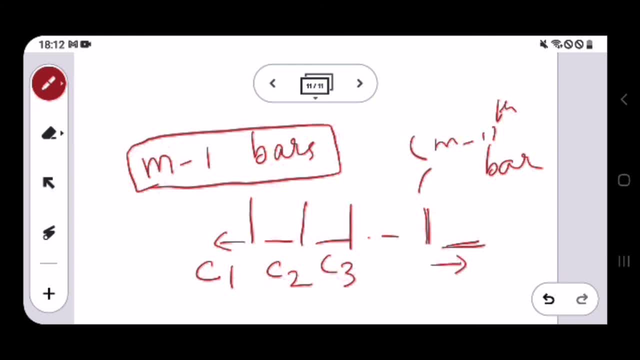 after that bar, whatever is coming, it represents the mth container. okay, cm mth container. whatever object, how many objects it has, it represents that. and how many identical objects are there? identical objects are n right, so we can just have n symbols denoting identical objects. let's say: 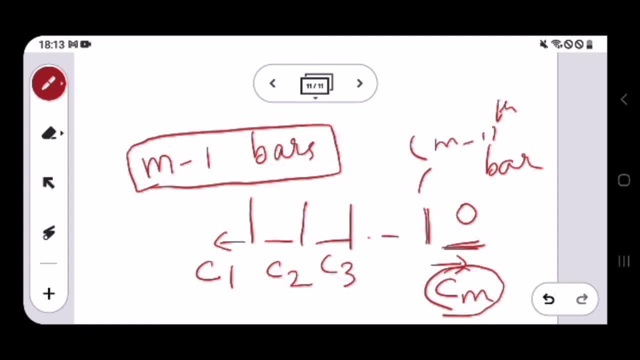 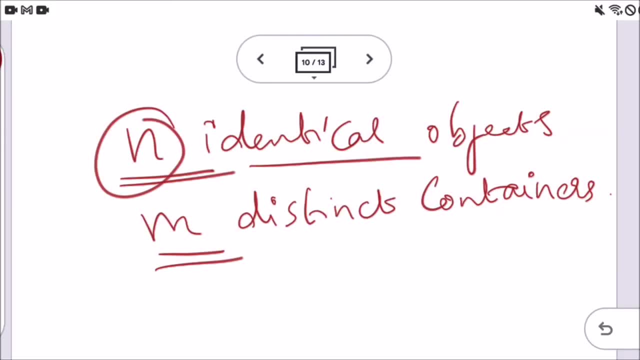 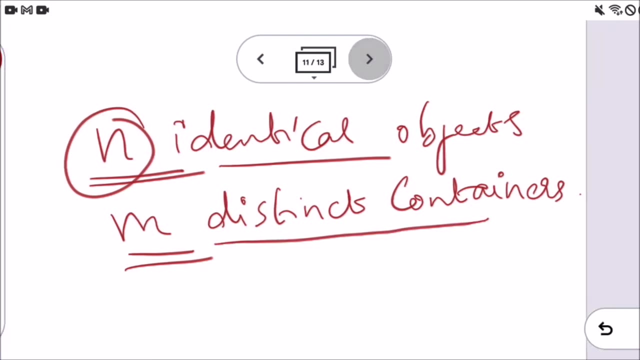 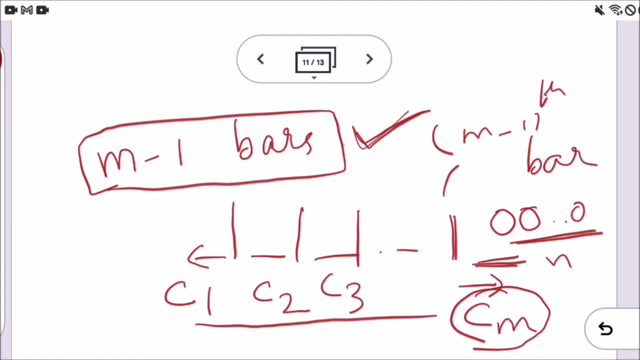 o is a symbol for the object here and there are n o's. okay, there are n o's, yeah. so we have n identical objects and m distinct containers. right, and because we have m distinct containers, we want to distinguish these containers. right, and that we can do using m minus 1 bars. right, so with the help of m minus 1 bars, we can actually 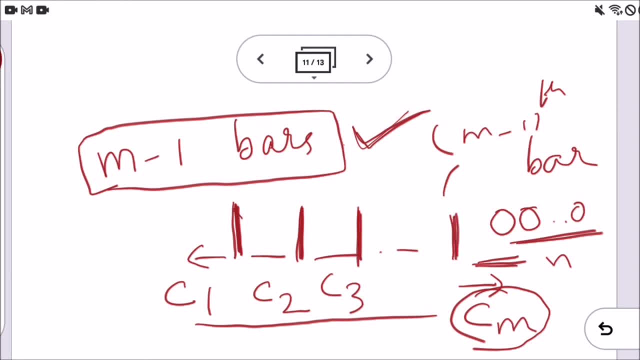 distinguish these m containers, because if you see, if you take the first bar, okay, and whatever is coming to the left of this bar, it is c1 container 1. okay, and so that if there are any objects coming here, let's say if there are like oh. 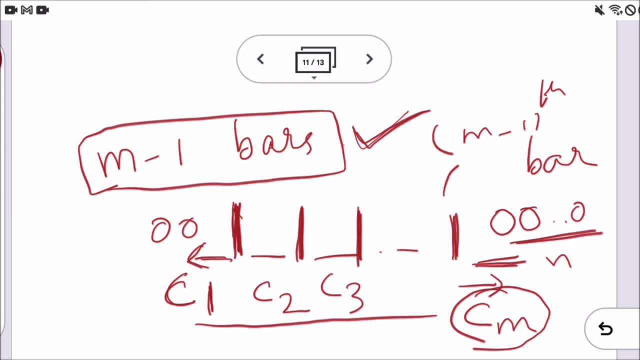 oh oh coming here, then it means that the if there are two o's coming here, it means that the container one have two objects, okay. and if say there is one o here, it means that c2 have one object okay. so c2 is the container which is coming in between the first bar and the second bar. 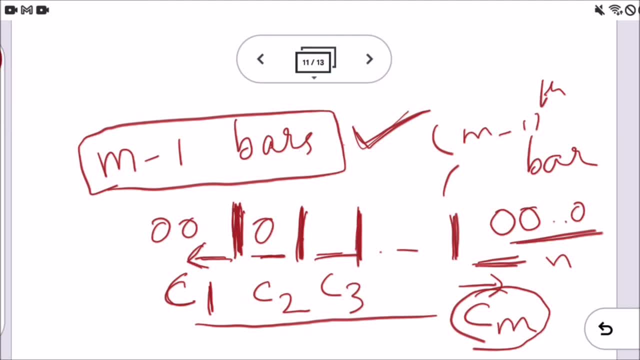 okay, and in between the second bar and third bar, we have third container and so on. so so this is how we distinguish the containers, using m minus one bars. okay, and any arrangement here. okay, so there are totally n identical objects, right, so each object, actually, we are denoting it by o, right, so there are n.